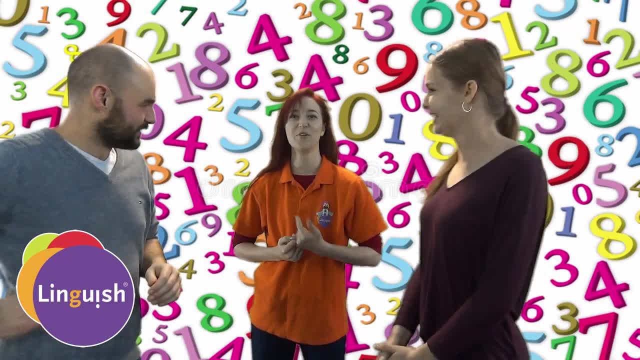 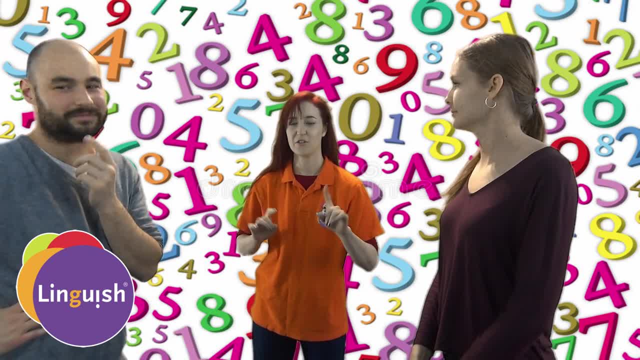 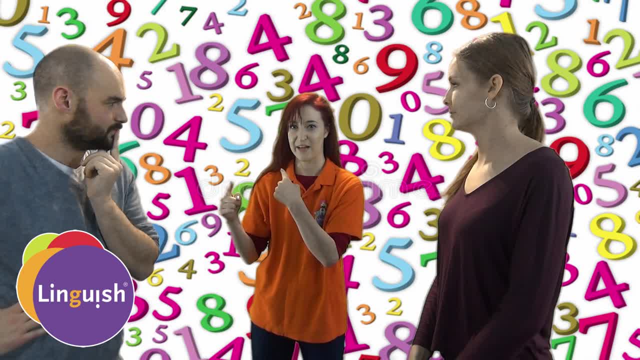 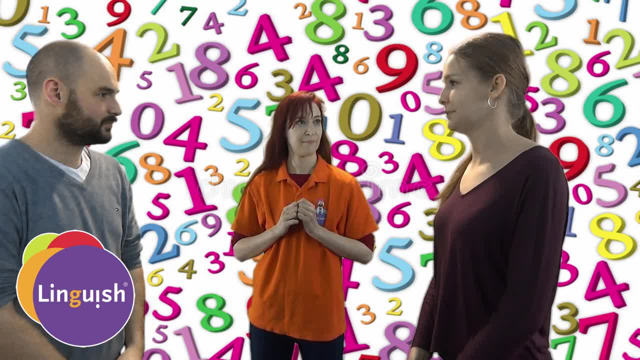 1,, 2,, 3,, 4,, 5., 1,, 2,, 3,, 4,, 5., 1,, 2., 1,, 2., 1,, 2., 2, 3.. 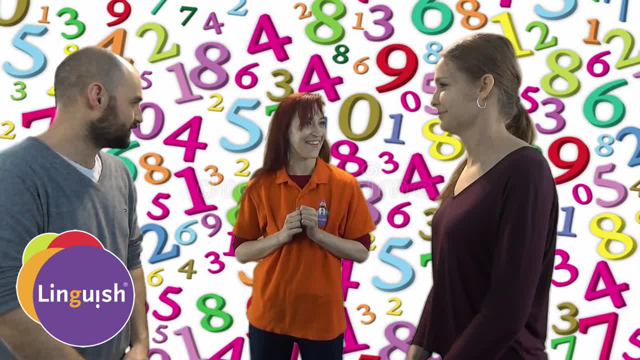 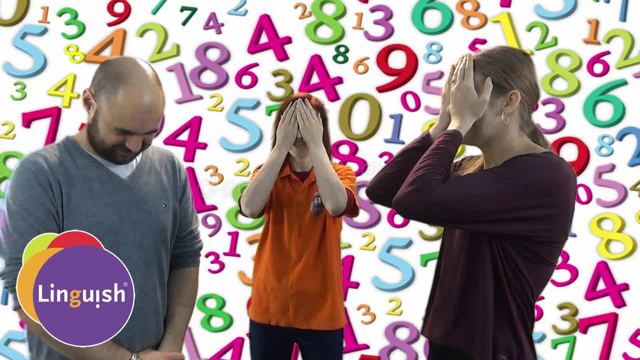 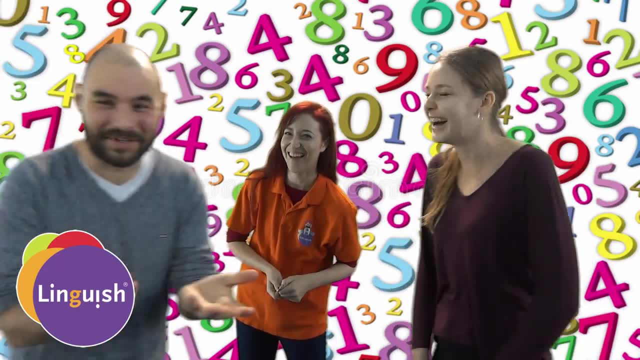 Oh, we did it Nice. And if you want to make it a bit more complicated, they have to do it with their eyes closed. Ready Go Like 9.. I could have stopped it, but I was like I'm just gonna say it. 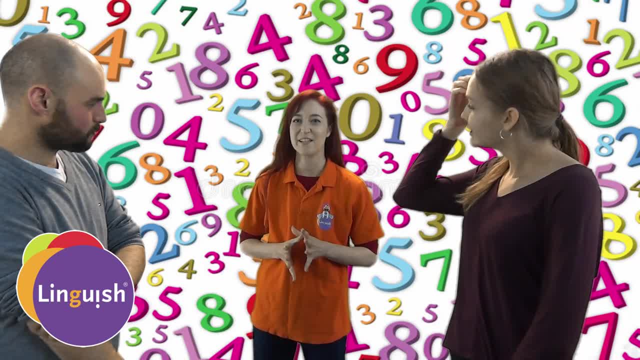 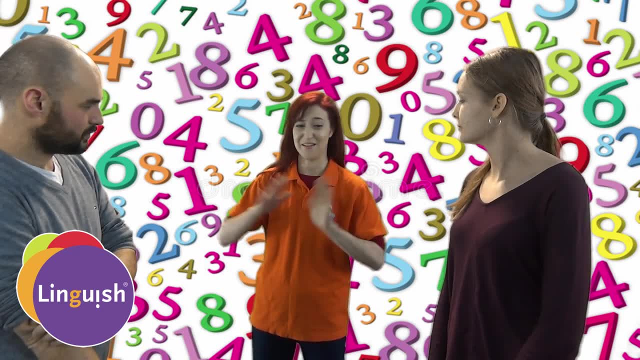 It works really well, especially if you have a really big group, because then everyone gets a chance to say the numbers And if they find it really easy, you can start making it higher numbers, from 1 to 15,, 1 to 20, it's up to you. 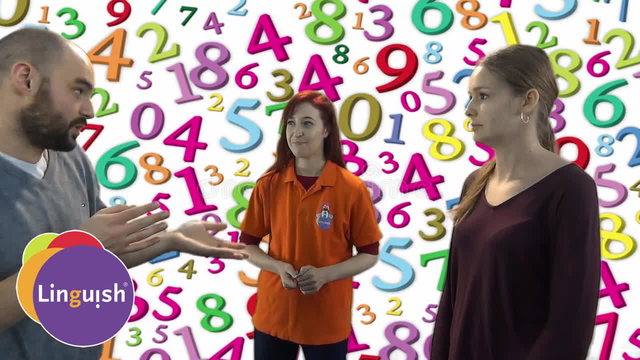 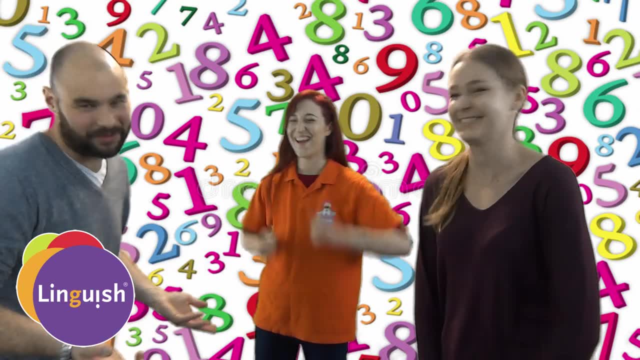 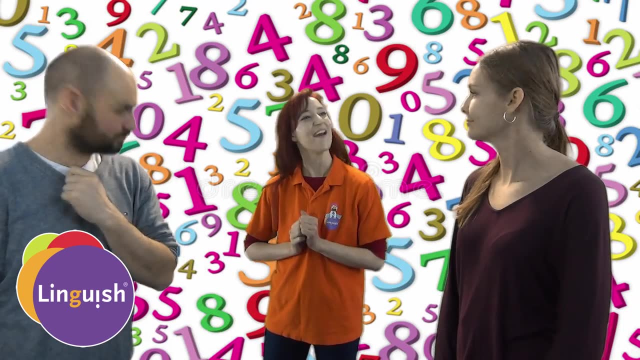 Can you also do it with, maybe the lyrics to a song they already know, Like Rudolph The Red Nose Reindeer: Yay, Yeah, completely, you can change any words that you want. Okay, hopefully you will enjoy this game. we enjoy it Next time. bye. Bye. 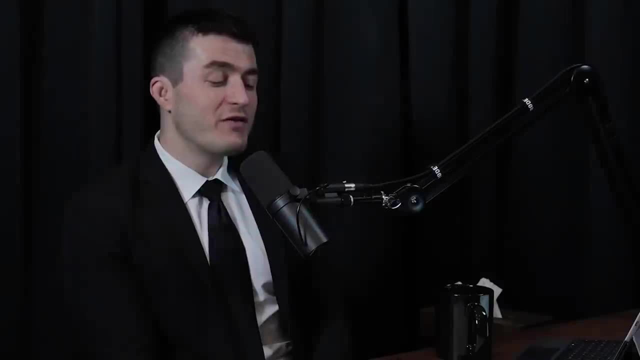 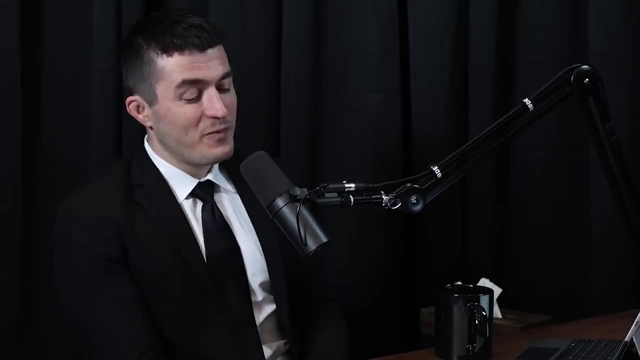 Can you give advice to young people in high school and college? Maybe they're interested in economics, Maybe they have other career ideas. What advice would you give them about a career they can have that they can be proud of, or a life they can be proud of? 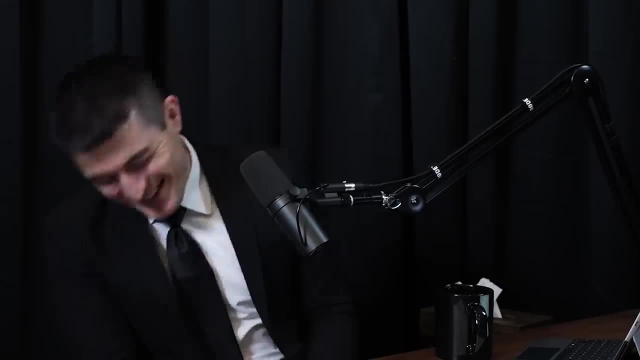 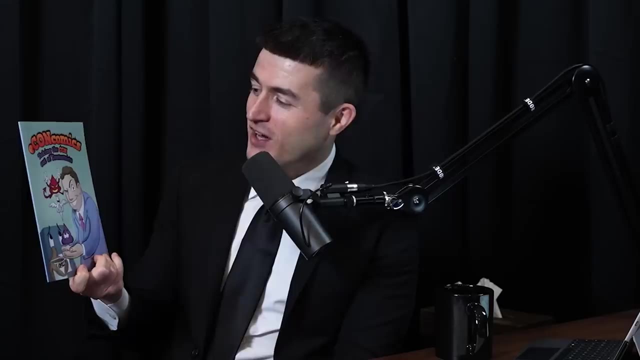 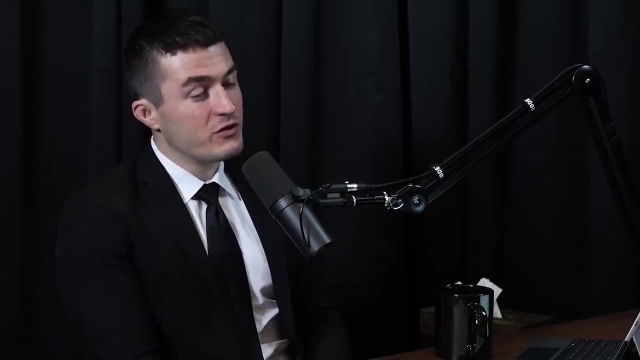 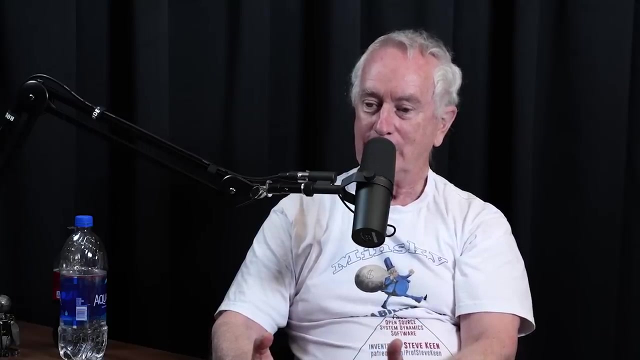 Mainly in a career. I say: don't do an economics degree. Okay, There's a little book on comics, Econ Comics, Taking the Con Out of Economics. They should start with that and then say: screw it to an economics degree. Yeah, because what you learn is an obsolete technology. Learning economics at a university. 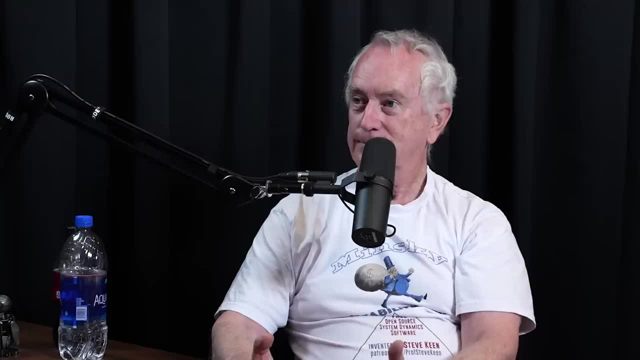 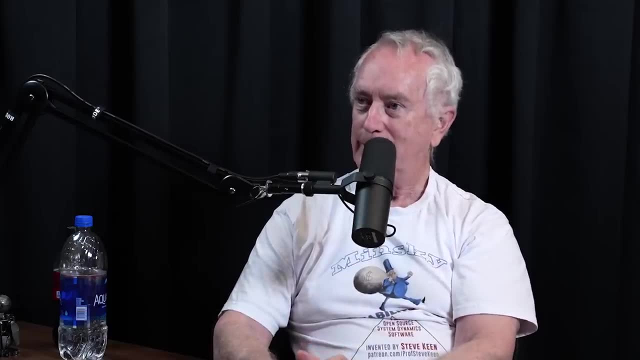 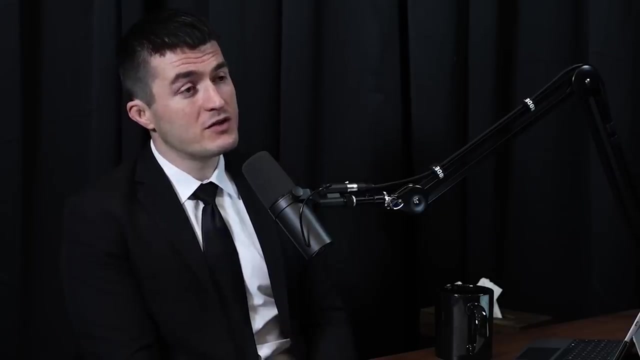 is like learning to make astronomy Earth-centric equilibrium epicycles being added to make your models fit the data. It's not that economics is not a discipline worth deeply studying. It's that economics at the university- education around economics- Is so bad.